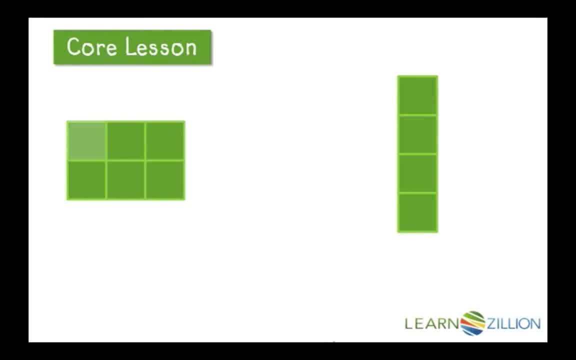 look at the area of the two. the rectangle on the left is an area of one, two, three, four, five, six square units that make it up. On the right, it's one, two, three, four square units that make that rectangle up. So, even though they 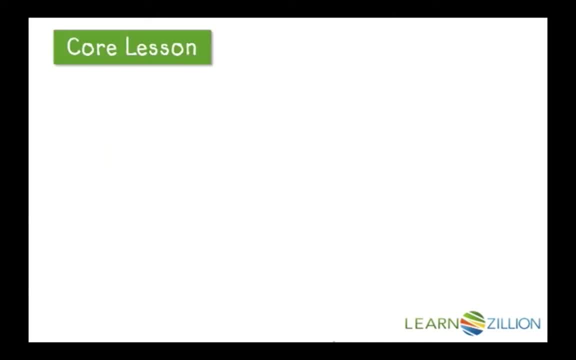 have the same perimeter. they have different areas because of their shapes. So let's look at this rectangle. It has a perimeter of 12 units, and I made two more rectangles that also have perimeters of 12 units. I'm going to 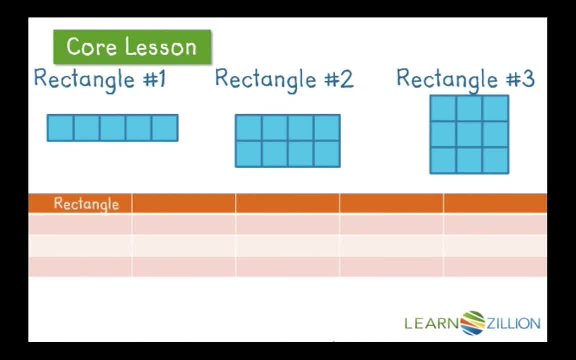 compare all of their measurements on this chart. So we'll look at the rectangle number, the perimeter, the length, the width and the area. So rectangle number one has a perimeter of 12 units, It is 5 units long and it is. 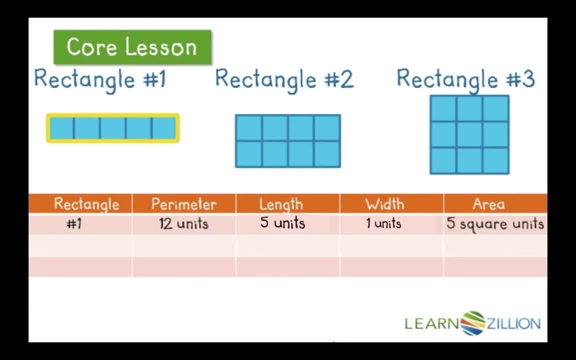 one unit wide And the area is five square units. Rectangle number two also has a perimeter of 12 units. It is 4 units wide, a long and units wide, and it has an area of 8 square units. Rectangle number three also has a perimeter of 12 units. 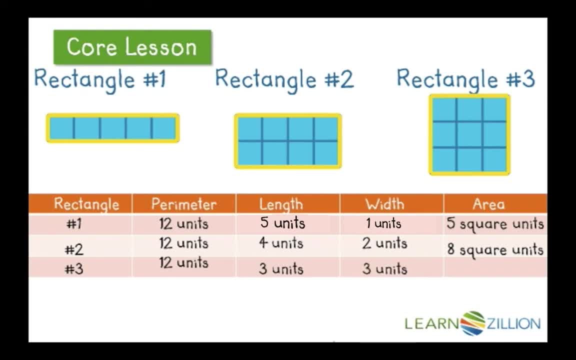 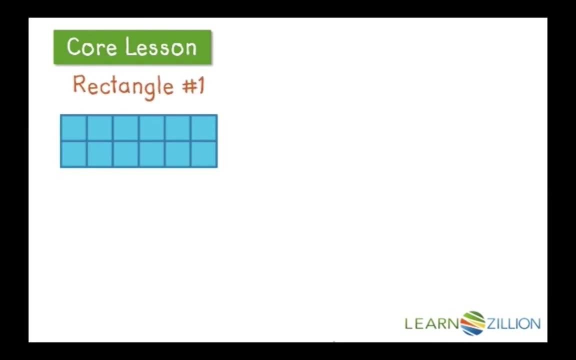 Its length is 3 units, its width is 3 units and its area is 9 units. So, even though they all have the same perimeter, they have different areas because they are different shapes. Let's go back to that rectangle we saw at the beginning. I made three more. 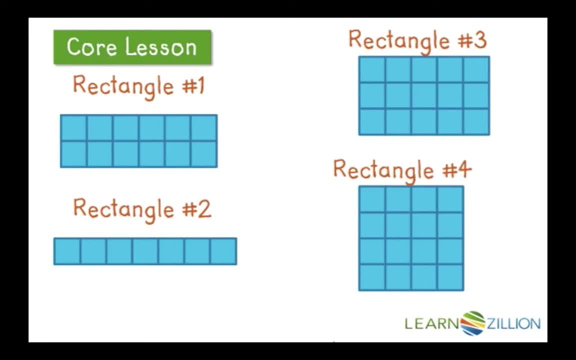 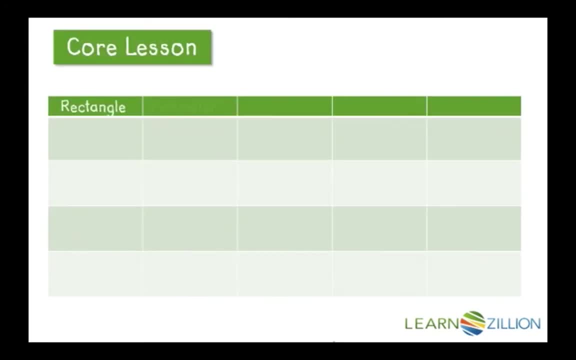 rectangles that all have the same perimeter But because they're different shapes they have different areas. So now we're going to make another chart to help organize that information. Again, we have rectangle perimeter, length, width and area. So rectangle number one has a perimeter of 16 units. Its length is 6. 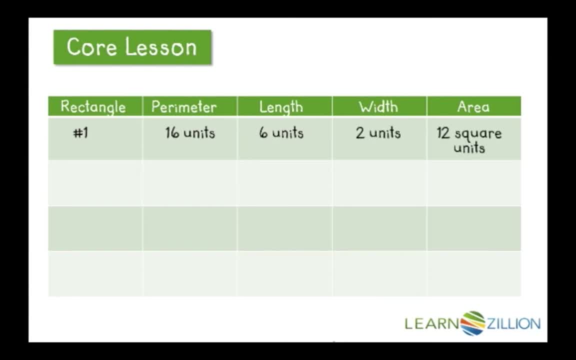 units. its width is 2 units and its area is 12 square units. Rectangle number two has a perimeter of 16 units, a length of seven units, a width of one unit and an area of 7 square units. Rectangle number three has a perimeter of 16 units as well a